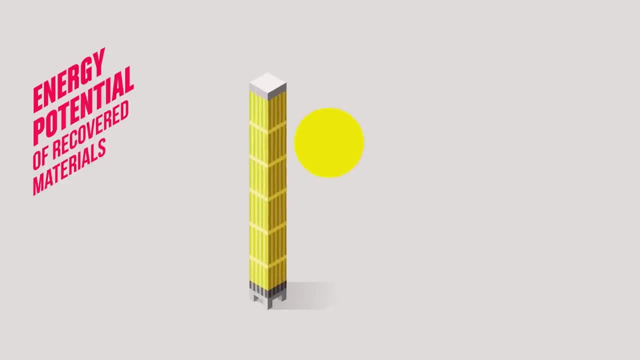 plutonium contained in the fuel, amounting to 96% of the nuclear material. The remaining 4% are the nuclear materials. This final waste is conditioned in a safe and sustainable way, as are the metallic structures, which are also non-reusable. 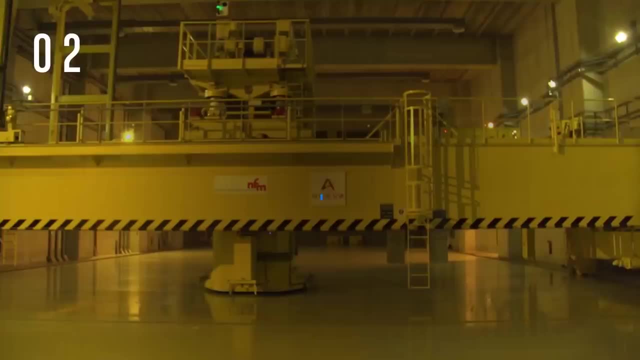 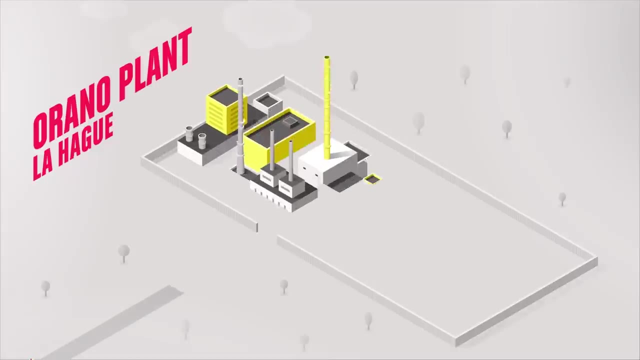 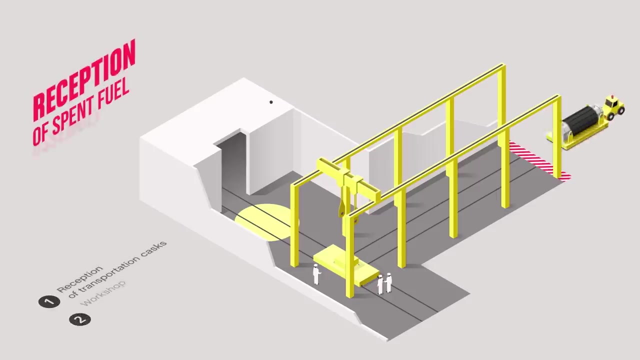 There are two tasks: The recycling of nuclear materials on one hand, and the optimum waste management on the other. Explanation: Used fuel assemblies are transported from a nuclear plant to La-Ague site in completely safe tasks. They are transferred to a first-working facility. 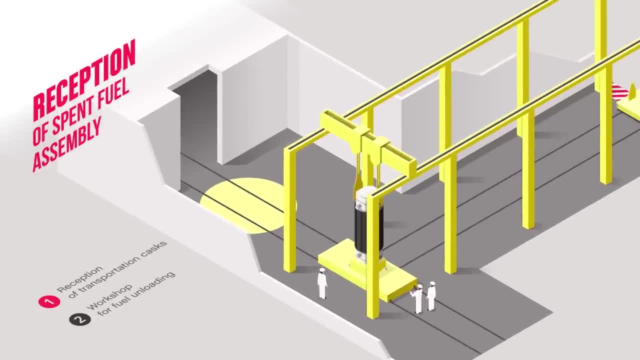 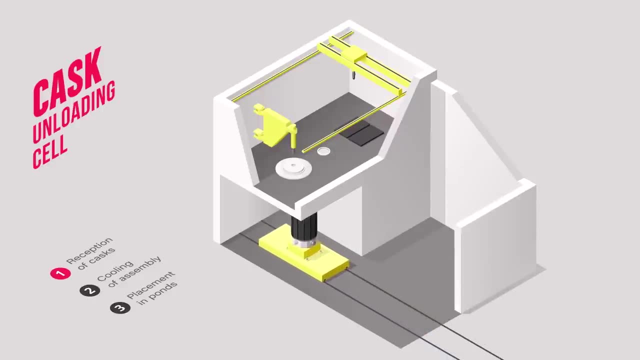 They are transferred to a first workshop for reception and storage in ponds. The casks are controlled, prepared and then docked with perfect tightness to the unloading cell. Here, as in all cells, complete and extremely reliable automation is used. The assemblies: 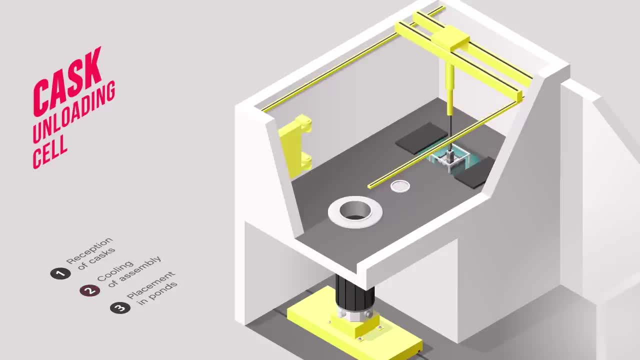 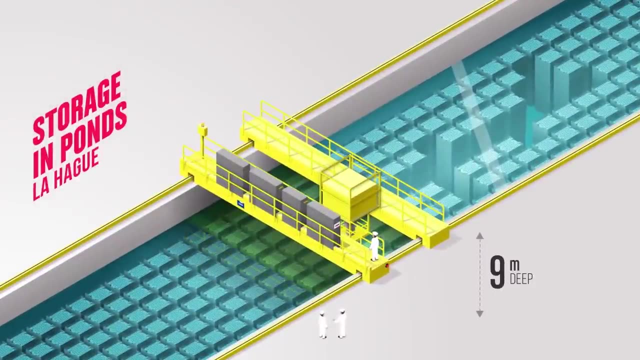 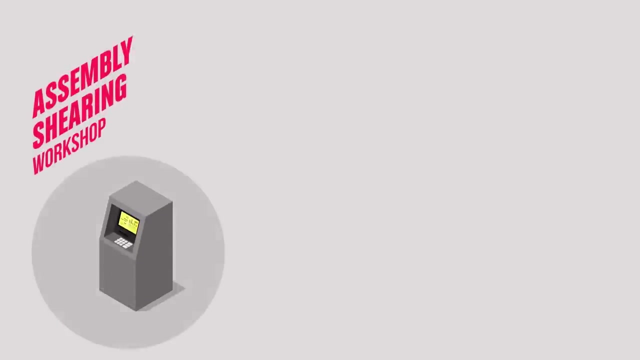 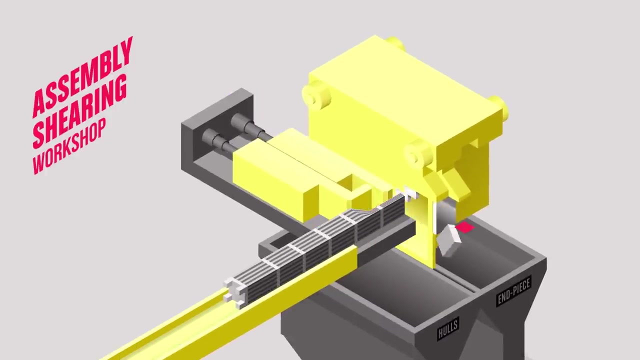 are unloaded, cooled, then placed in a storage pond to enable part of the radioactivity to decrease. After several years in the pond, an assembly is taken to a workshop where it will first be cut, a process known as shearing. The end pieces are removed. As for the cladding, which contains the recyclable materials, it 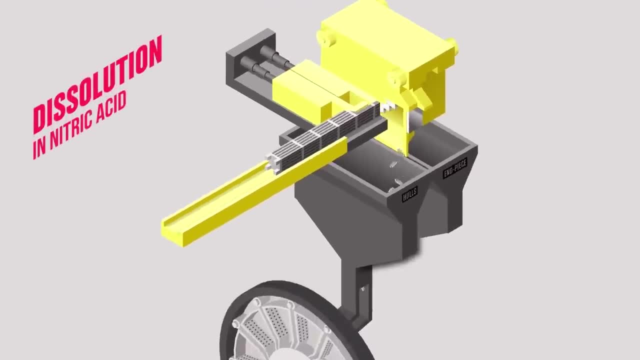 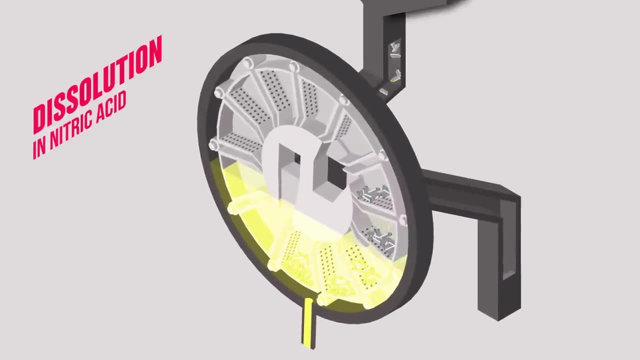 is sheared into 35mm sections. The dissolution step allows the recovery of the material contained in the sections for treatment. The dis-solution step allows the recovery of the material contained in the sections for treatment Inside the dissolver. the sections are plunged into nitric acid. 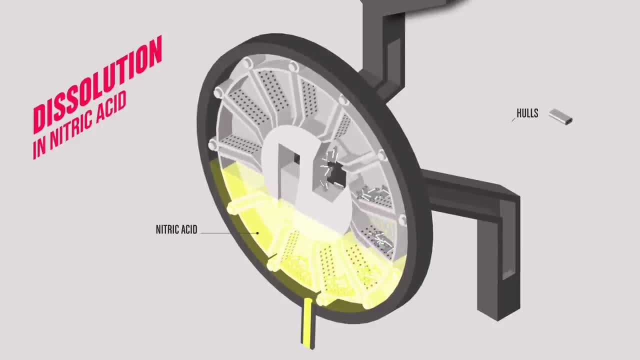 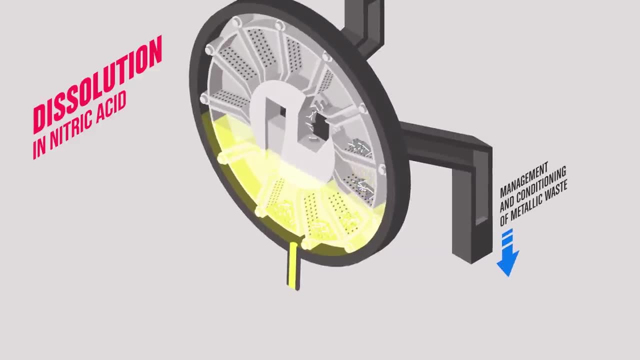 The result? On one side, sections which have been emptied of their material, which are called hulls. The hulls then follow the same treatment line as the end pieces, the same line used for metallic waste. On the other side, nitric acid containing uranium, plutonium and fission products. 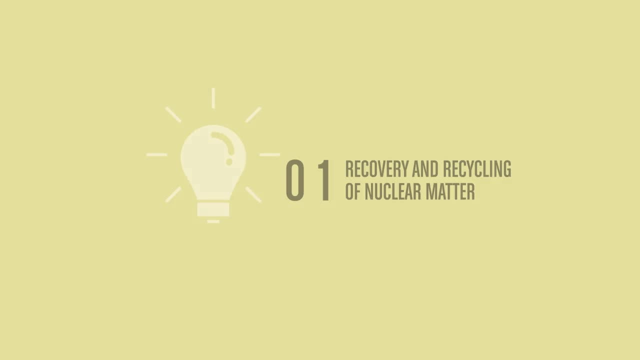 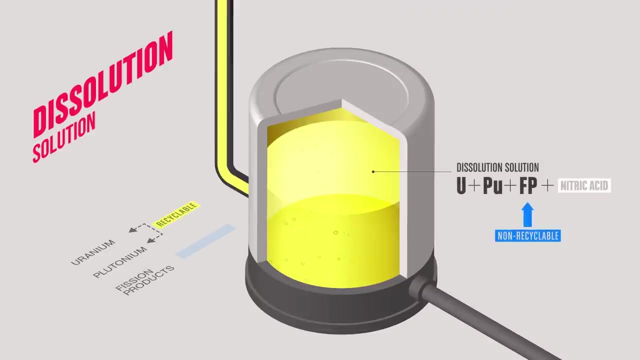 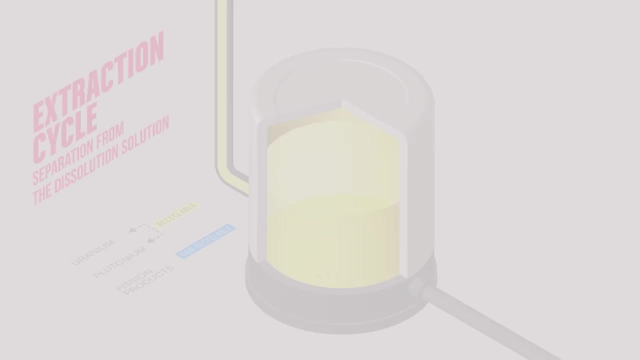 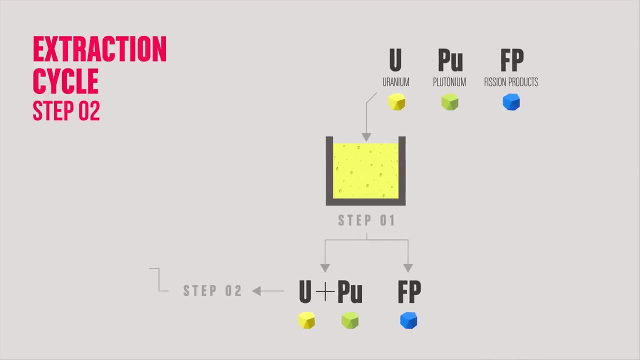 The solvent therefore contains recyclable uranium and plutonium and non-recyclable fission products. The extraction step consists in separating these three materials in two phases. Firstly, the fission products are separated from the plutonium and uranium and secondly, the uranium. 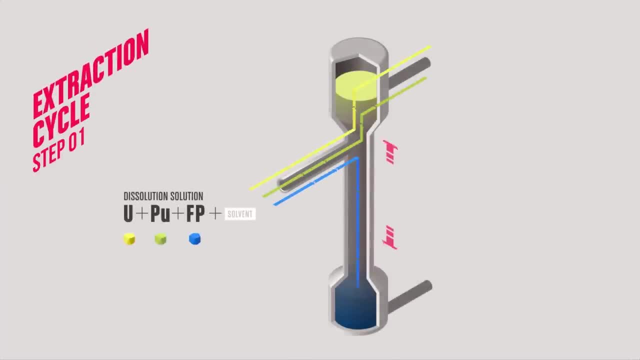 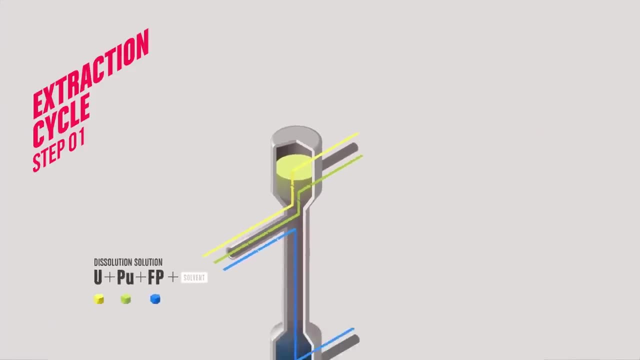 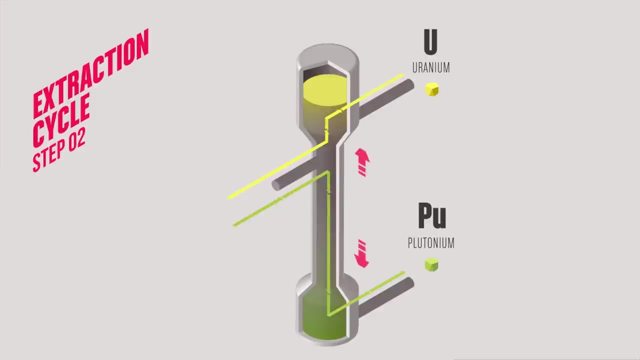 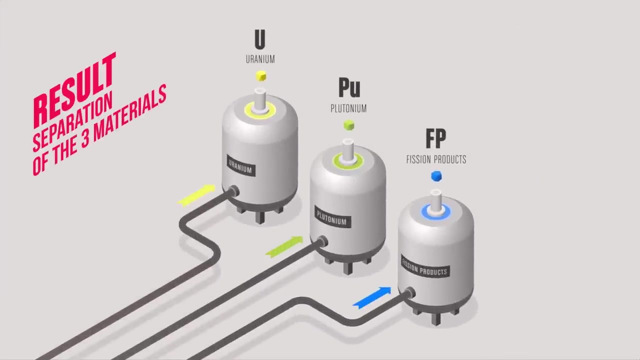 from the plutonium. Extractions are carried out in the liquid phase. A solvent is used for one element to have an affinity to an organic phase, while the other remains in liquid phase, Like water and oil. the two elements separate naturally At the end of the extraction cycles. three separated materials are obtained. 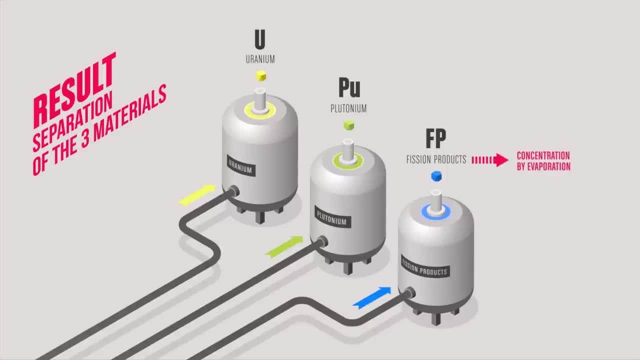 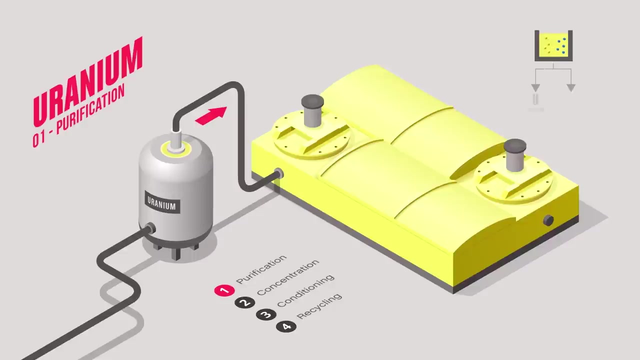 The fission products concentrated by evaporation, Uranium also concentrated by evaporation, And plutonium, which is transferred to the liquid phase. This is transferred to its workshop for conditioning. The uranium is first purified. This involves removing the last traces of the fission products. 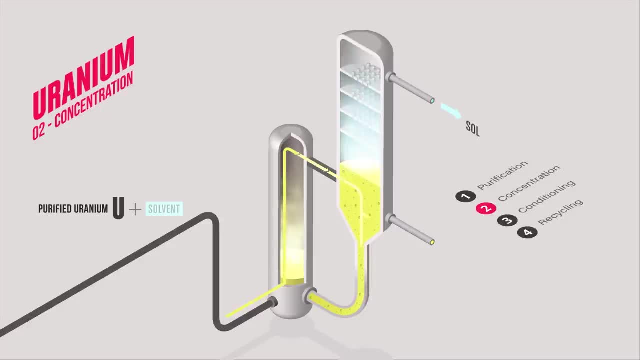 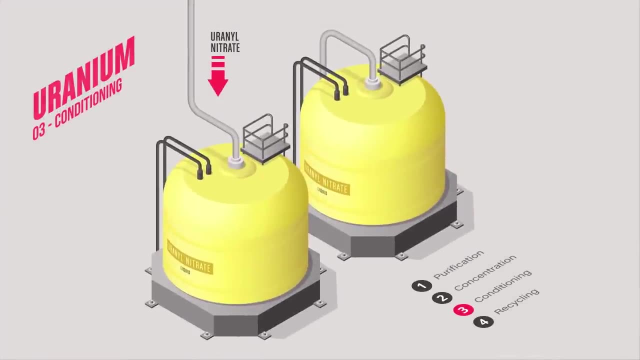 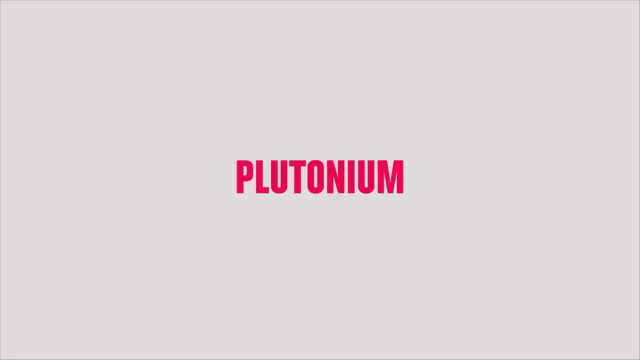 Then it is concentrated in liquid form, called uranyl nitrate, to be recycled again in the fuel cycle. The uranyl nitrate is then stored in tanks before being shipped to be recycled in enrichment and fuel manufacturing plants. Plutonium contains a large quantity of energy. 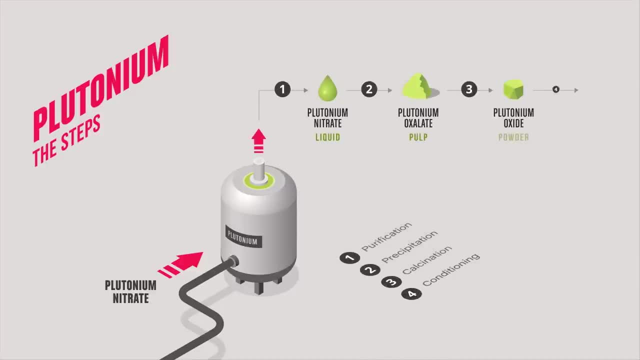 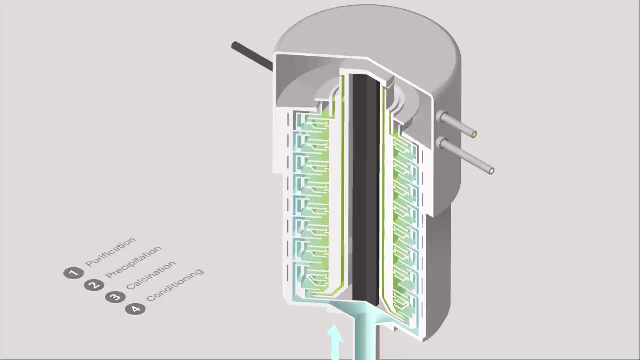 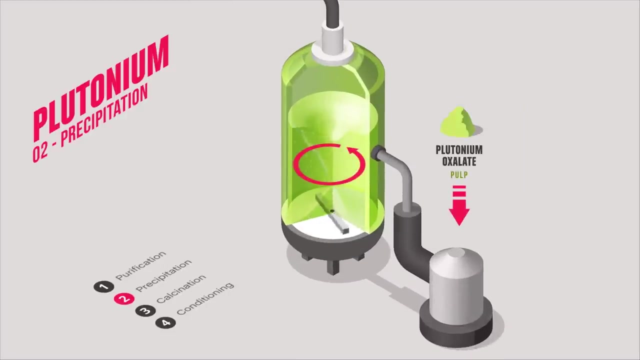 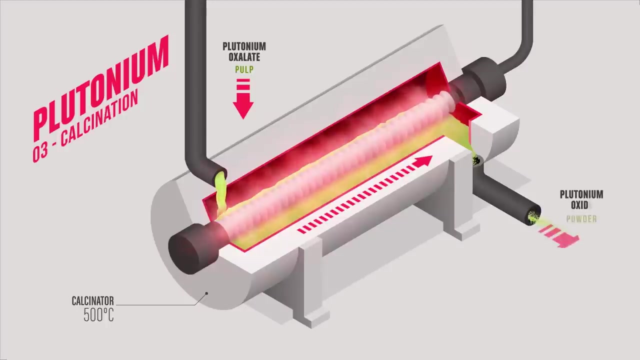 Its treatment consists in changing it from a liquid form to a solid form. For this it is first purified, then converted into plutonium oxalate, a pulp using precipitation. Calcination then completes the transformation of the oxalate into a powder. 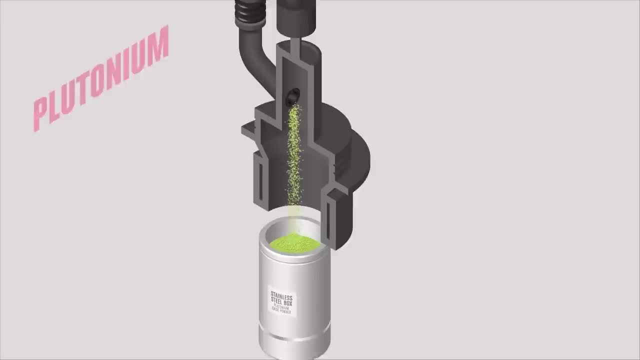 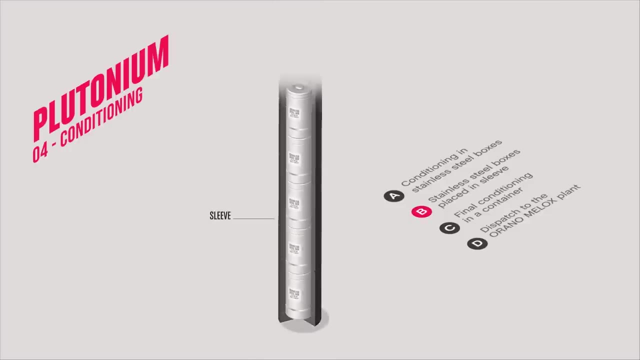 called plutonium oxide. The plutonium oxide is finally conditioned in stainless steel boxes which are placed in cases, which in turn are placed in containers. Particular attention is given to the air tightness and non-contamination of the containers. After a storage phase, they are sent to the Arana Melox plant. 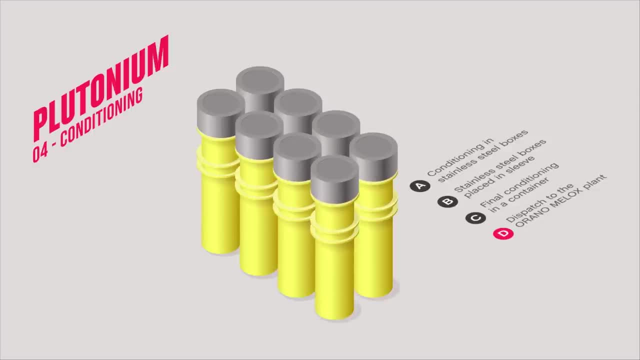 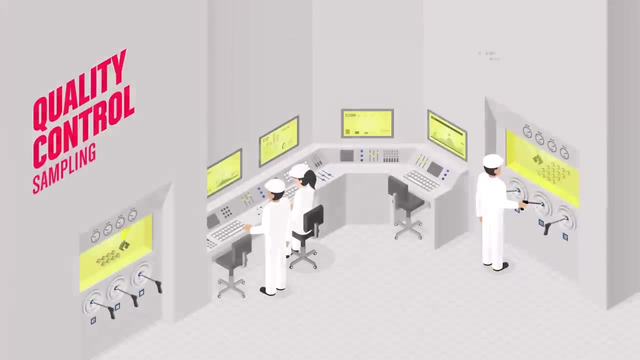 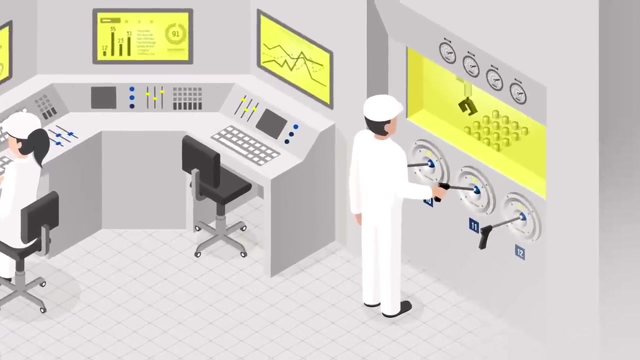 which makes new fuels called MOX In nuclear power plants. MOX fuels are used to generate electricity. At each step of the process, the quality of the products is meticulously analyzed. At Orano La Ag, the purity of the materials obtained is systematically measured. 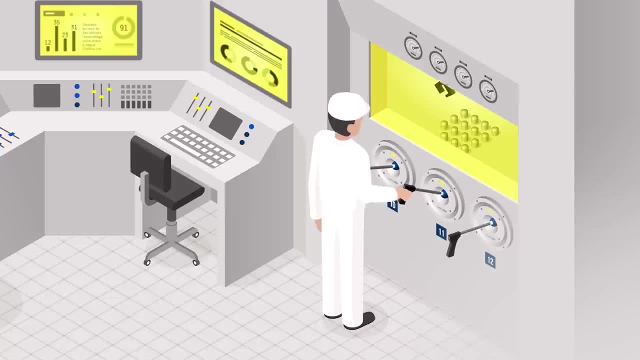 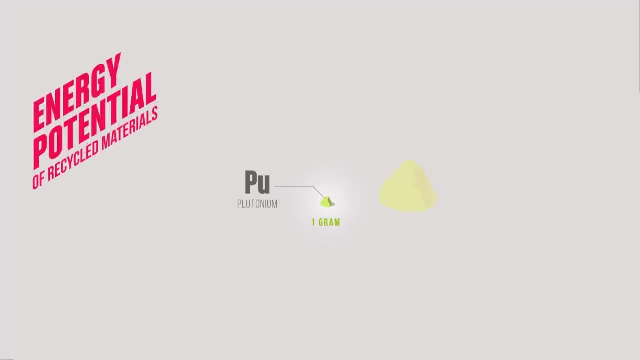 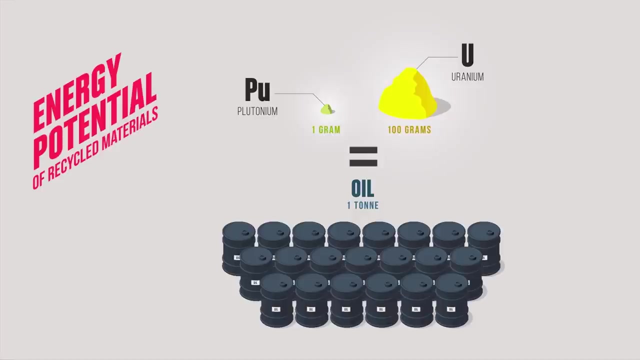 by chemical, physical and isotopic analyses. Materials recycled at Orano La Ag have a considerable energy potential. One gram of plutonium, which equals 100 grams of uranium, represent the energy equivalent of over one metric ton of oil. The amount of lithium in plutonium oxide is estimated to be about 1.5 times that of uranium. 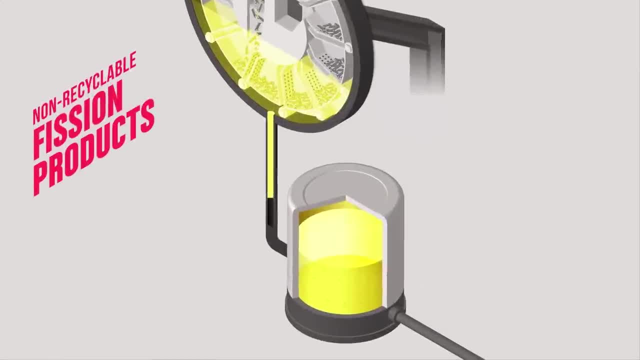 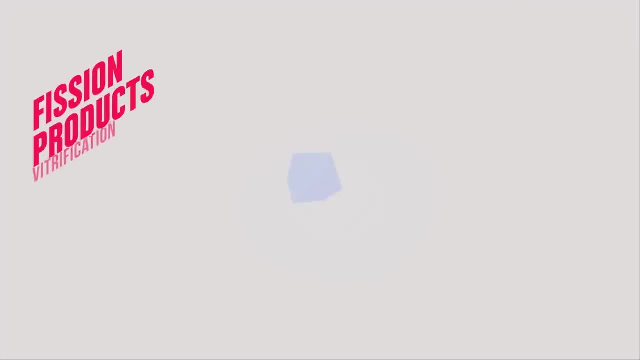 Fission products extracted from the solvent are not recyclable. They contain almost all of the used fuels' radioactivity. They are incorporated in glass frit and conditioned into an extremely stable form for optimized and long-term safety management. This process is called vitrification. 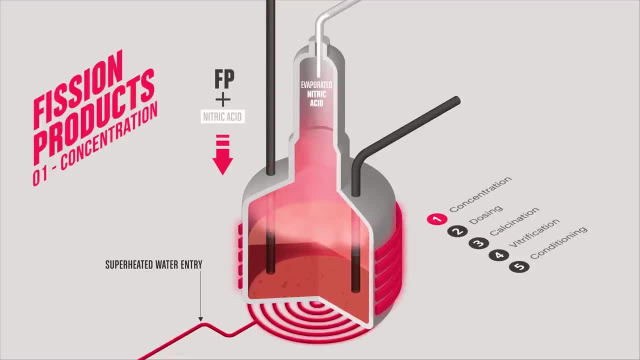 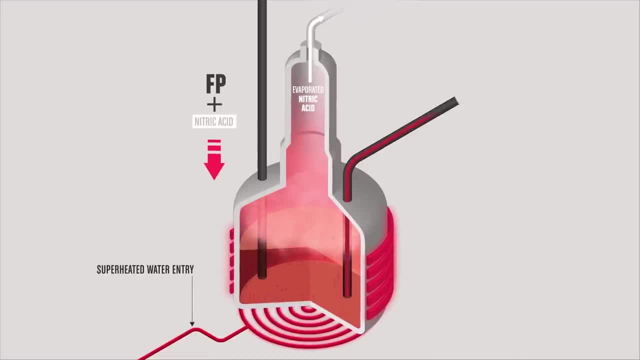 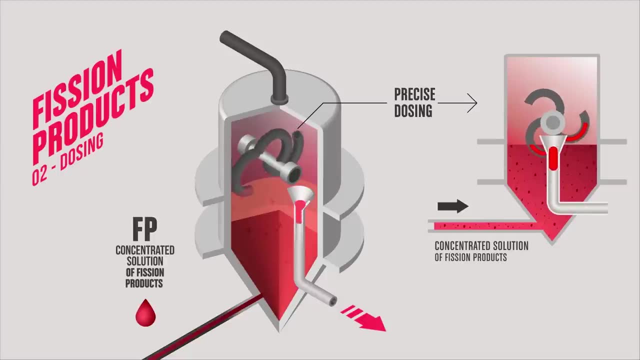 Evaporation of the Nitric Acid and Nitrogen. Evaporation of the Nitric Acid and Nitrogen: What's up in the left-hand vision? · Try to find hard-to-Bonel products that also contain nitric oxide. · For example, the. 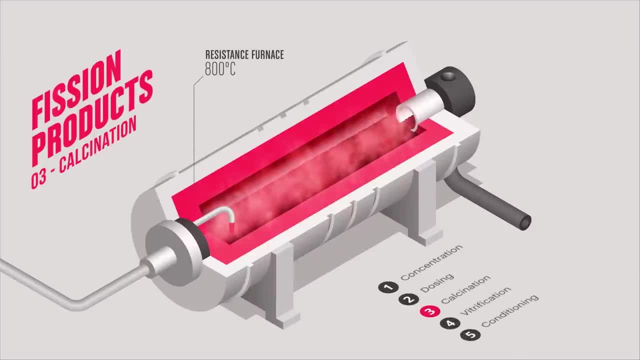 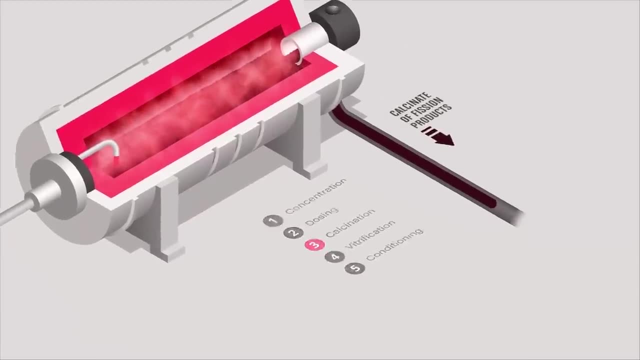 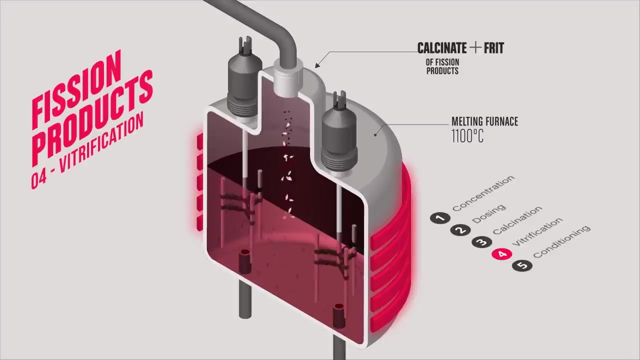 · Dis Warning · Saving. · Which Li Echo · Which Ziron? · Which Z marine? · Which Raining? · Which COO · Which BAE. The mix falls into a melting furnace heated to 1,100 degrees Celsius, which ensures the perfect incorporation of the products and a homogeneous glass form. 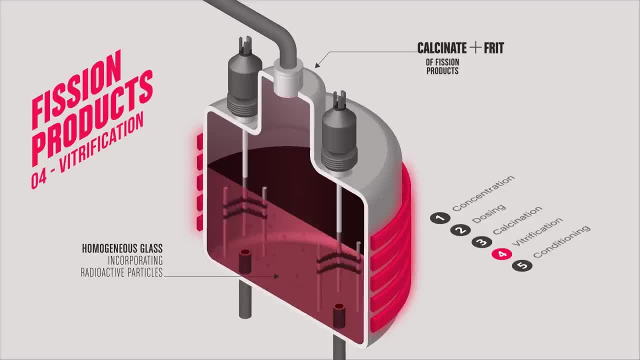 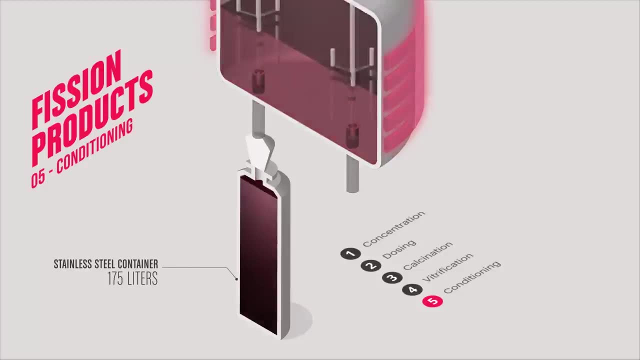 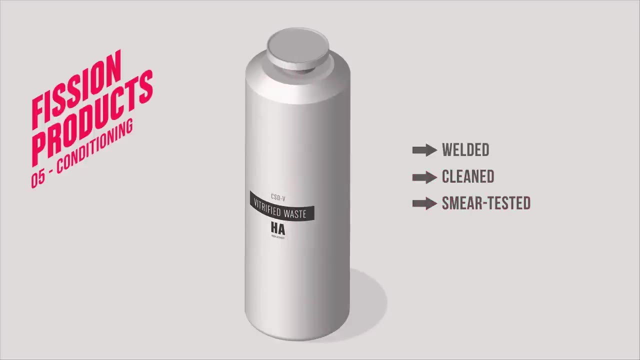 This guarantees a very chemically stable matrix for several tens of thousands of years. The molten glass obtained is poured into a 175 liter stainless steel container, which is then cooled, welded shut, cleaned and smear tested to check it is contamination free. 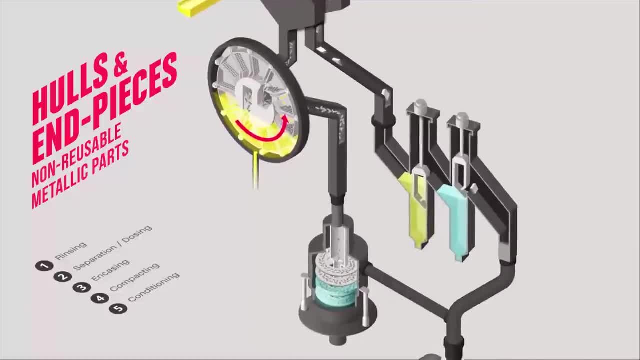 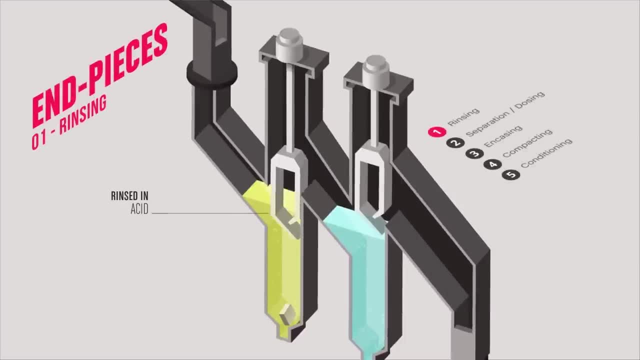 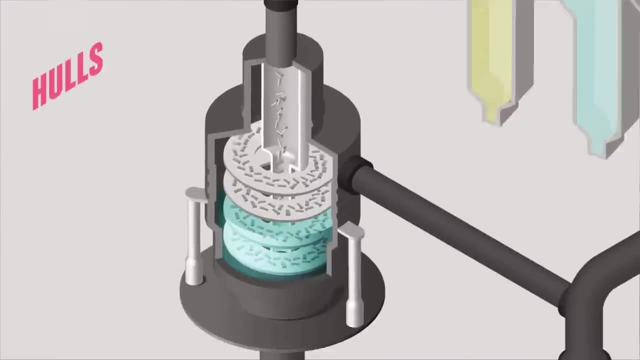 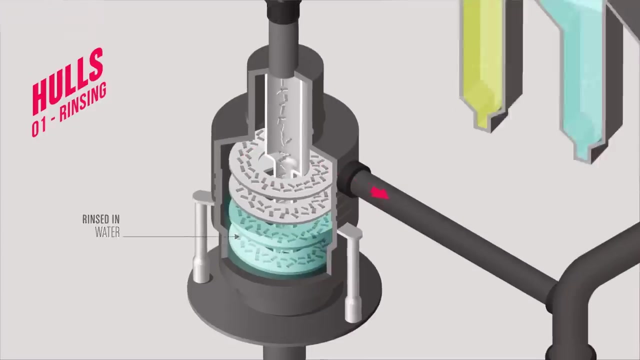 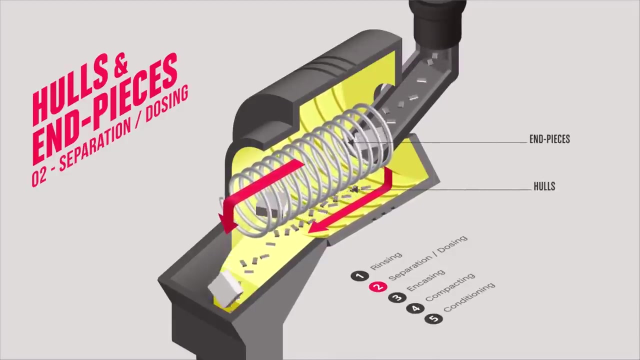 Regarding the metallic structure of the fuel assembly, the hulls and end pieces are rinsed separately. The end pieces in acid and water, the hulls in water Transported together. the hulls and end pieces are rinsed separately. The end pieces will then be precisely sorted by a separator doser.